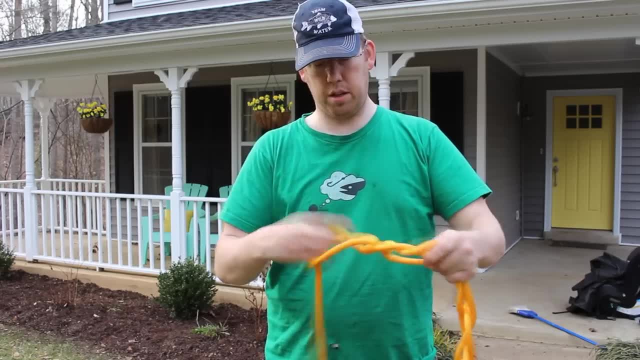 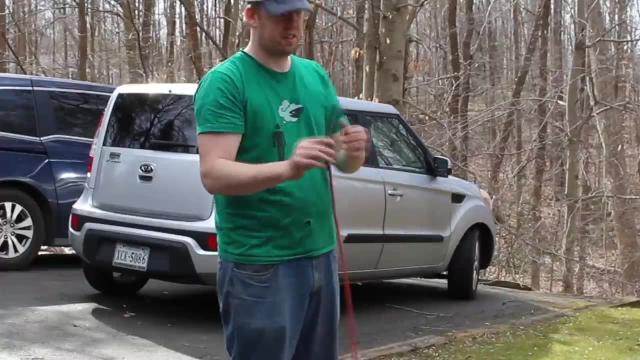 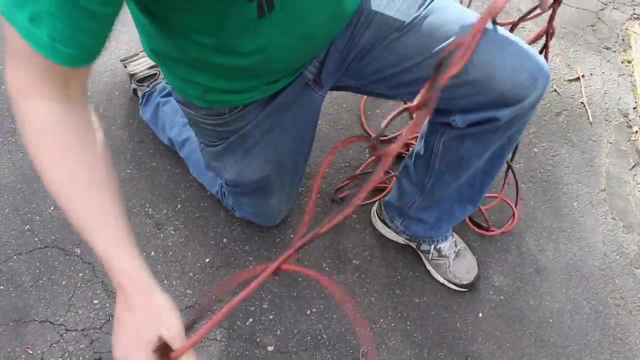 When you're done, You just go back and recreate the daisy chain, Start back where you left off. If you're going to do the daisy chain with an electrical cord, Start with the male prong And then work your way down. This hundred foot extension cord goes down to about 30 feet. 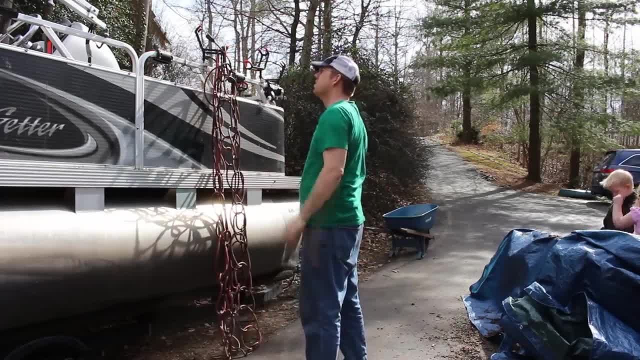 Hang it up on the wall And keeps it out of the way. So easy to use. You pull out as much or as little as you want. Just re-tie up when you're done. Now if you're in a situation where you need an adjustment. 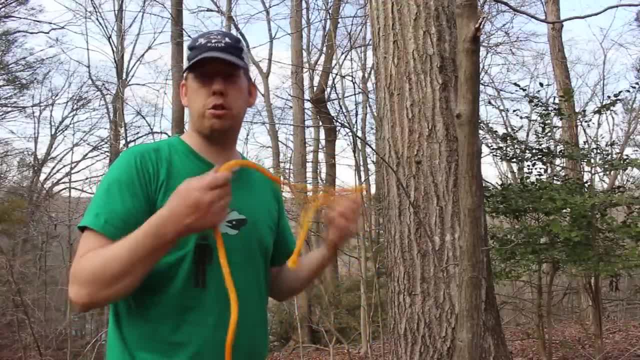 Now if you're in a situation where you need an adjustment. Now, if you're in a situation where you need an adjustment, You need an adjustable length of rope, Like you're stringing up a tarp or putting up a tent. We were often taught in Boy Scouts to use the tautline hitch. 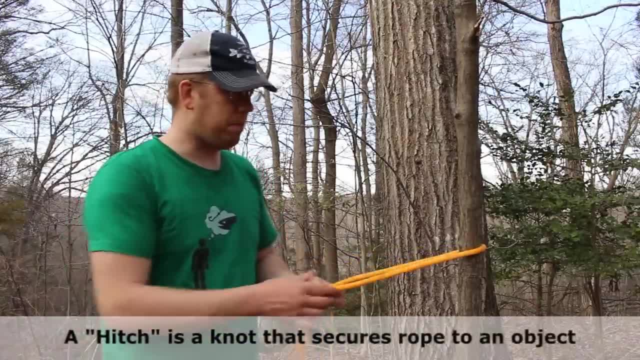 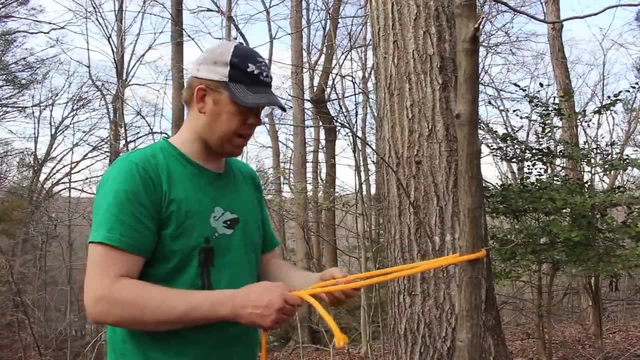 Or the midshipman's knot as it's called. But I've got something better, And the reason why it's better is because it's faster, Not just it's not faster to tie, It's faster to take down. So this right here is the Farrahman's friction hitch. 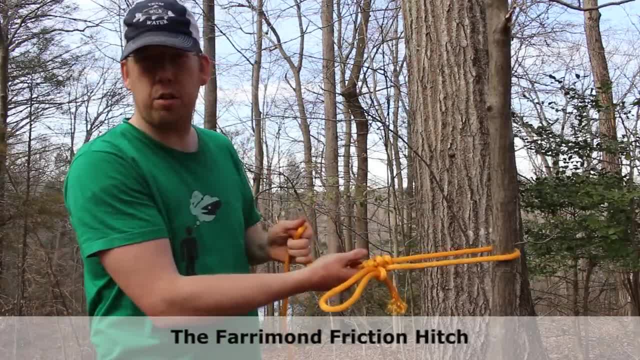 It's a little bit stronger than the tautline hitch or the midshipman's friction hitch. It's a little bit stronger than the tautline hitch or the midshipman's friction hitch. It's a little bit stronger than the tautline hitch or the midshipman's friction hitch. 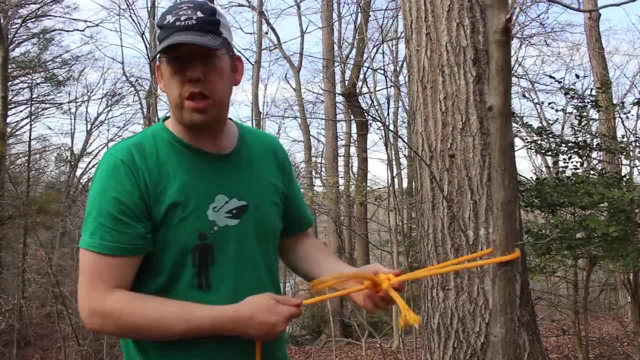 You can put more force on it without the loop closing. You can put more force on it without the loop closing, But the real advantage is that it's so easy to take apart. But the real advantage is that it's so easy to take apart. 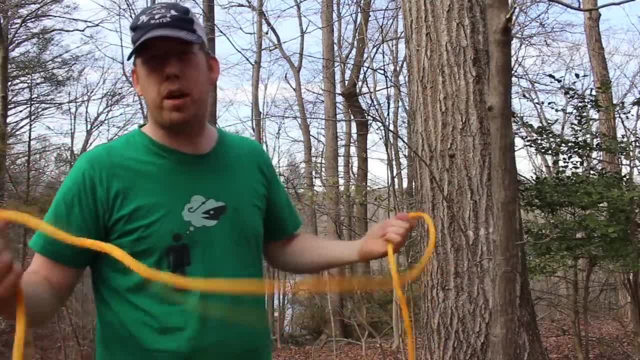 But the real advantage is that it's so easy to take apart. So it's time to break down camp or take that tarp down. So it's time to break down camp or take that tarp down. It takes seconds. This knot allows you to adjust the length of a rope by adjusting the size of the loop at the end of the rope. 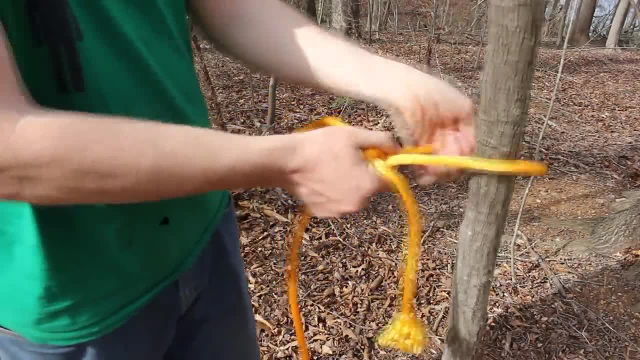 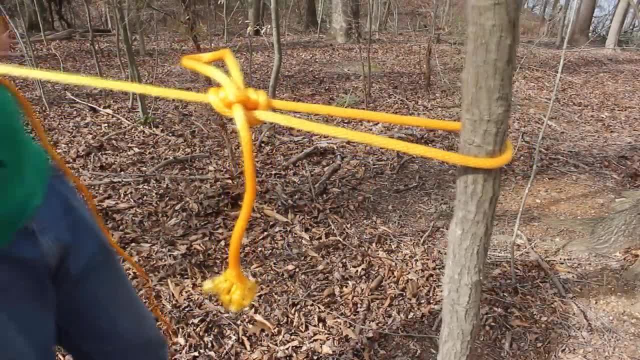 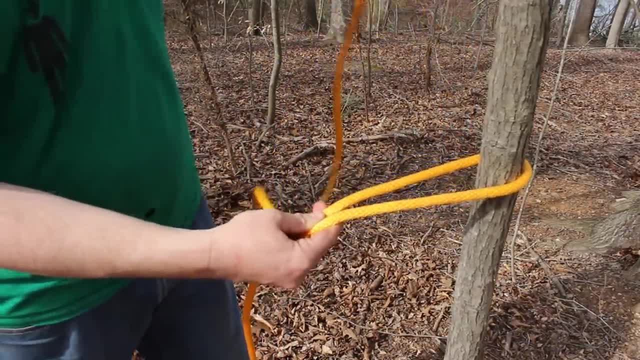 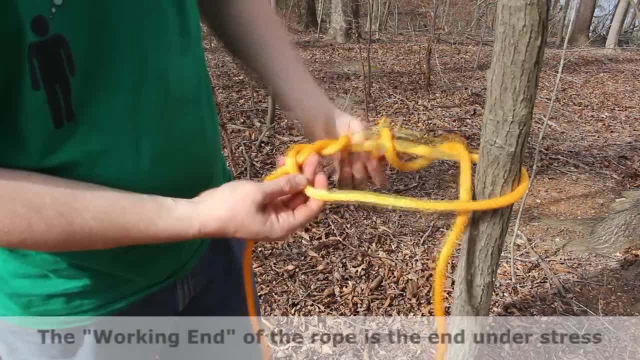 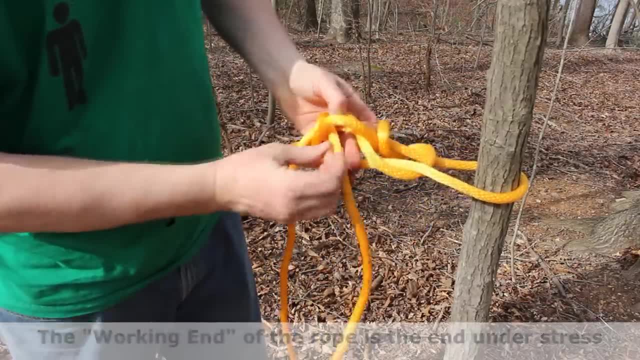 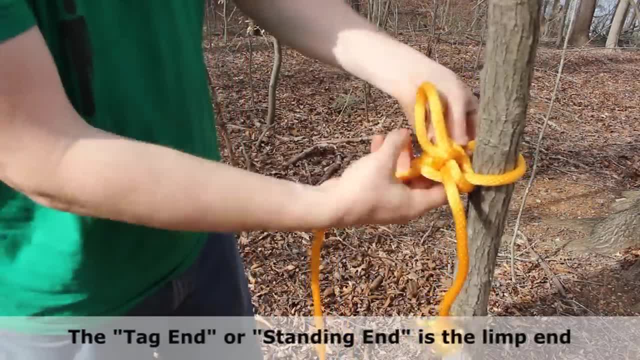 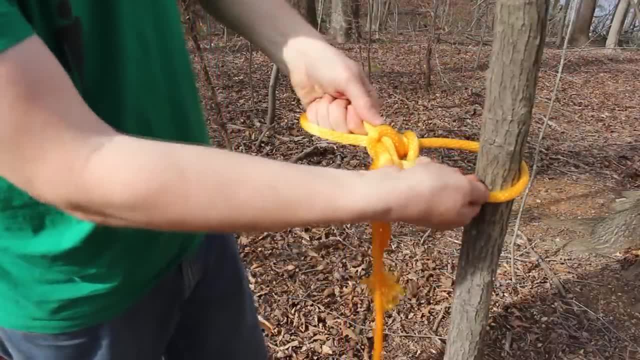 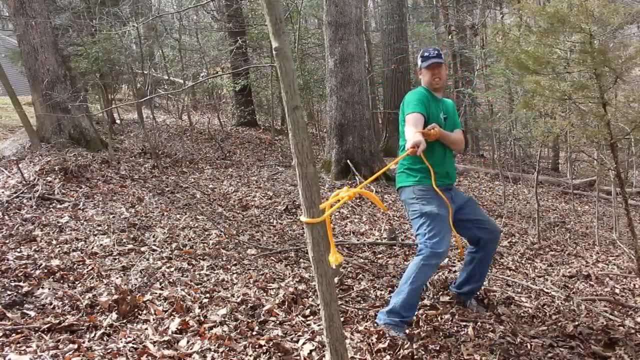 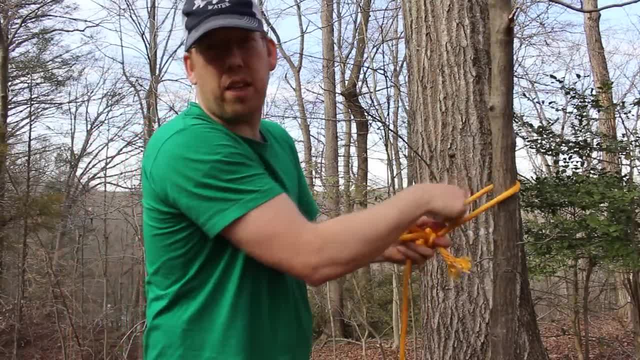 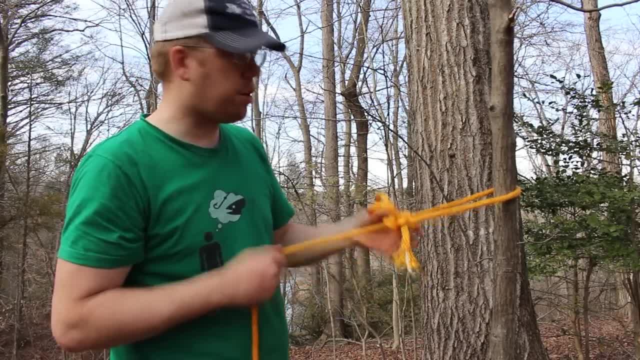 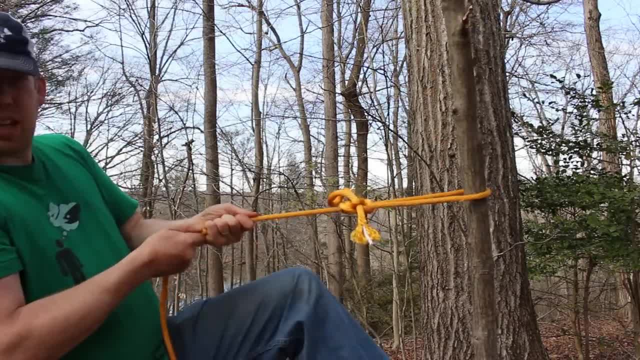 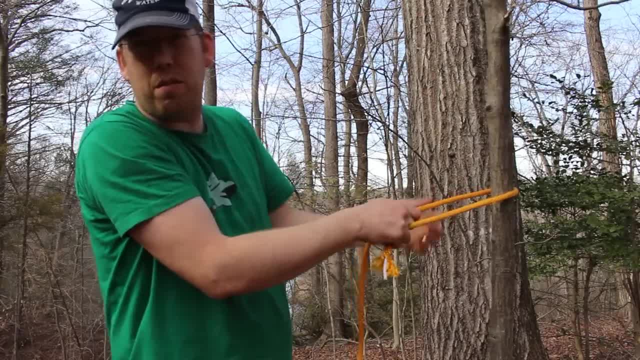 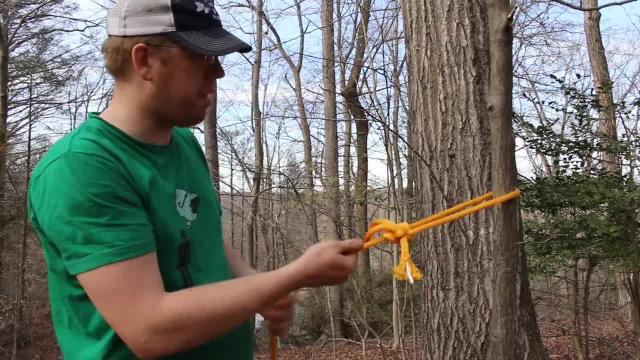 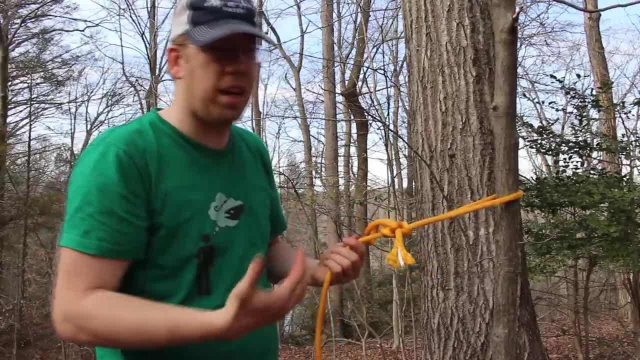 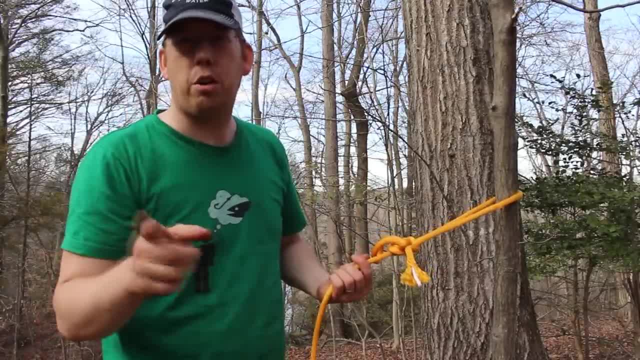 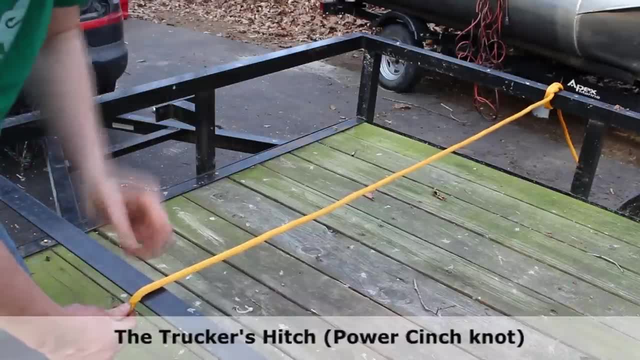 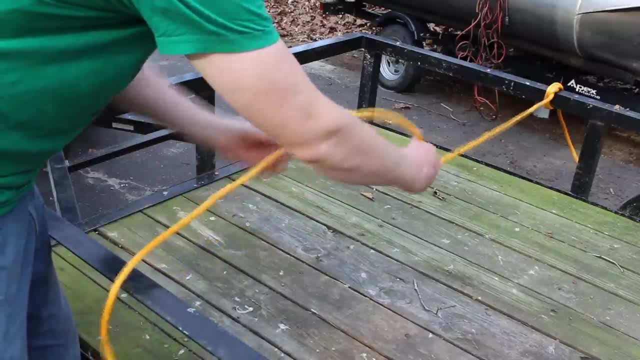 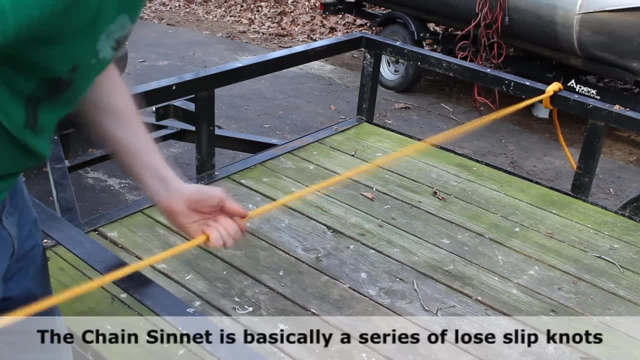 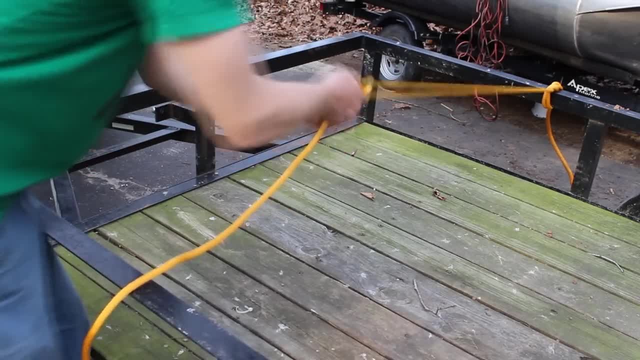 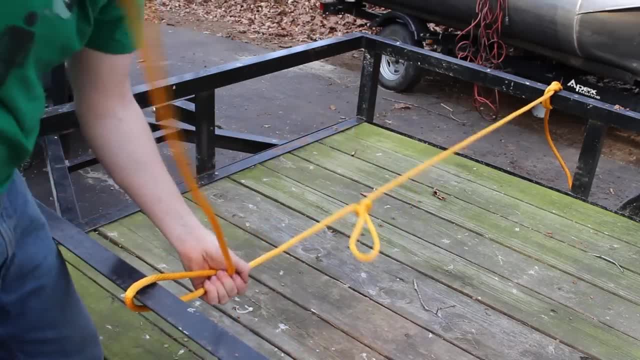 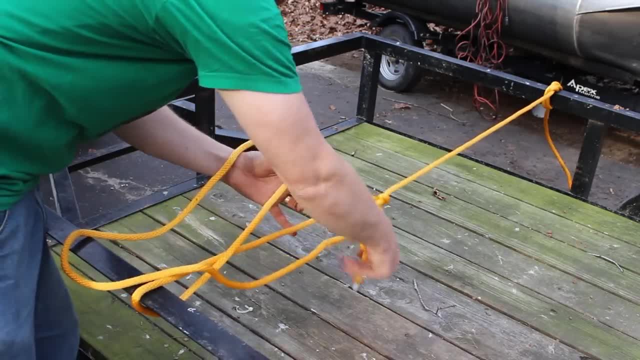 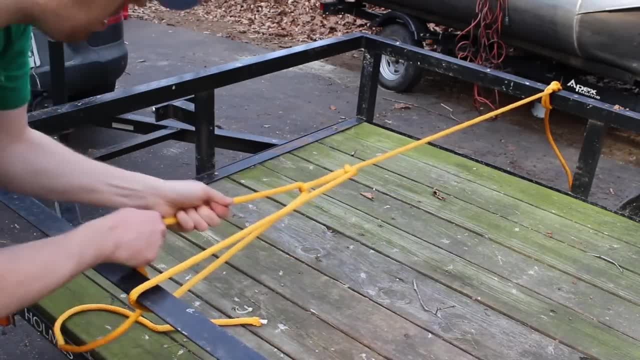 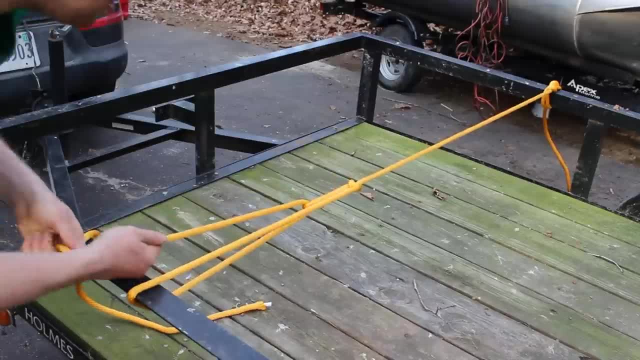 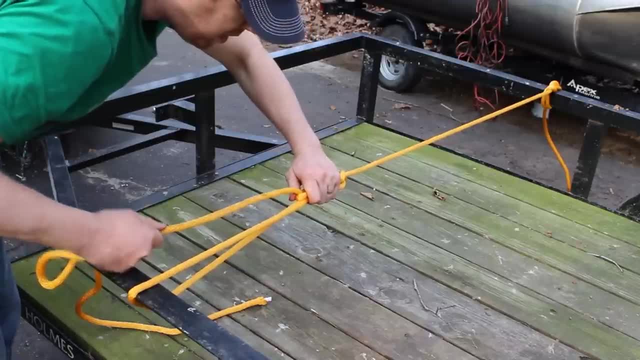 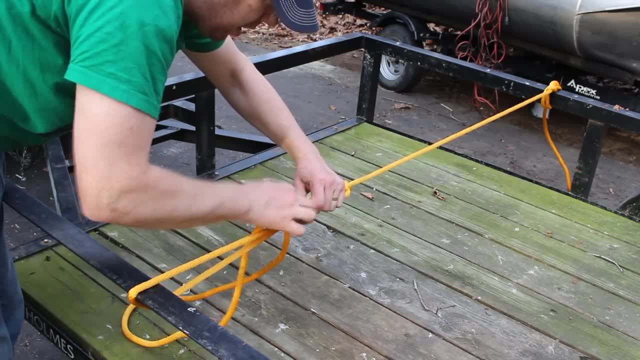 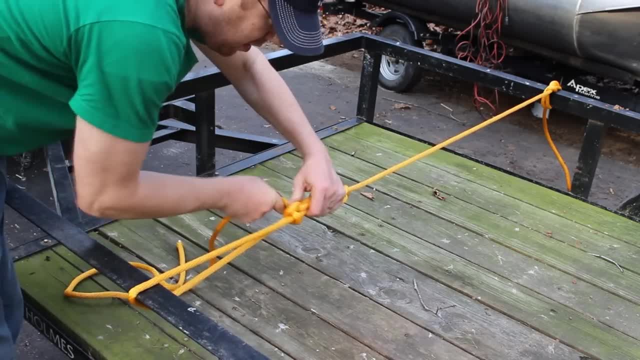 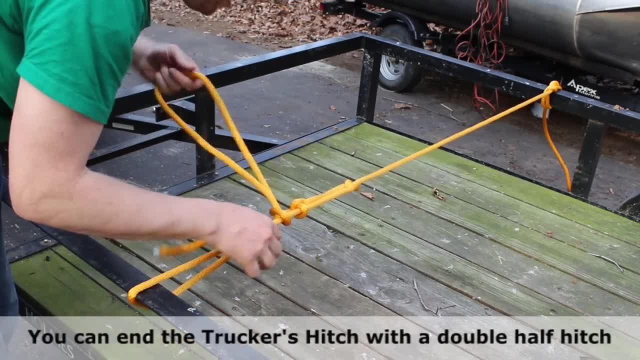 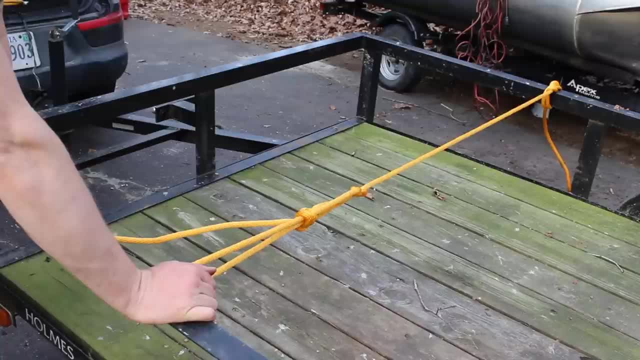 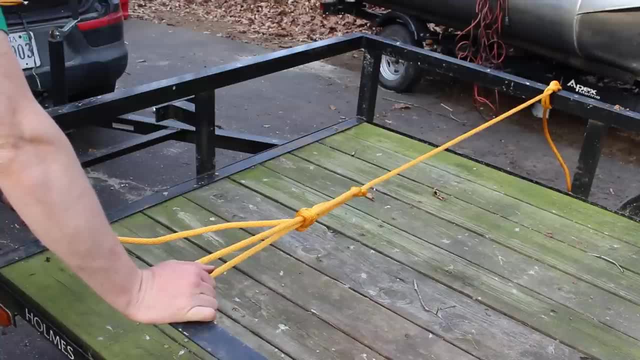 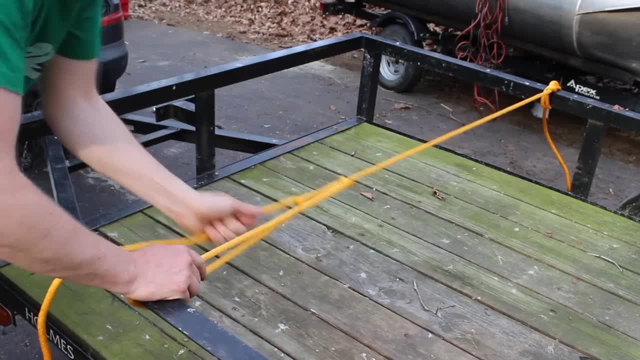 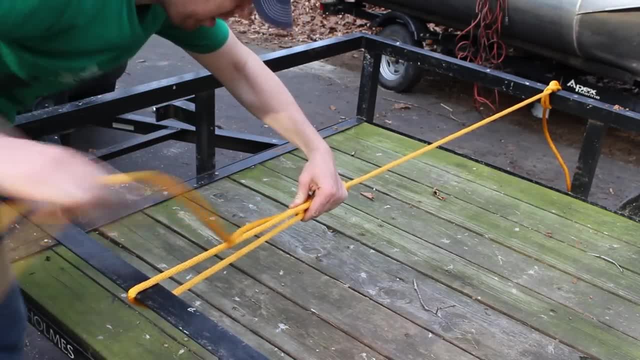 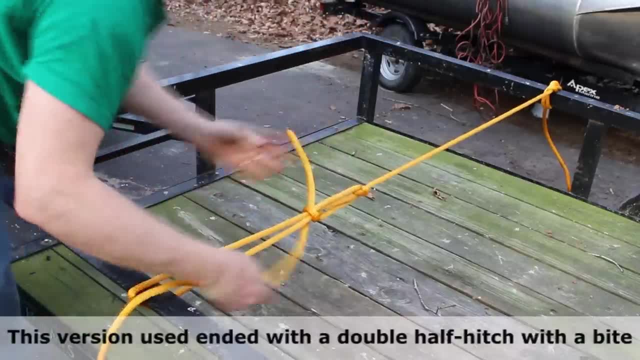 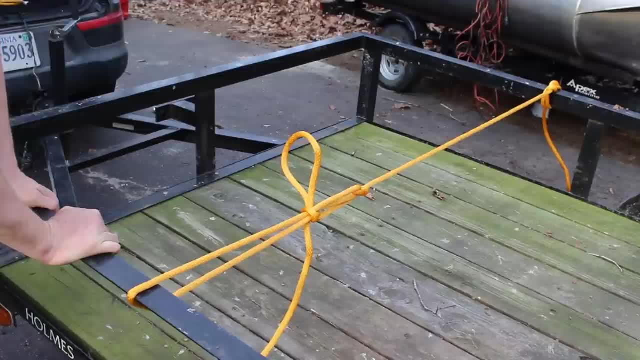 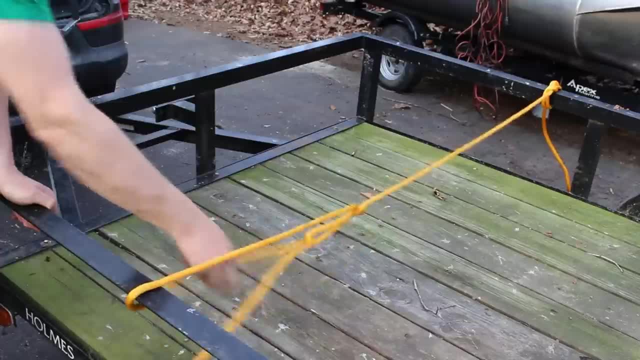 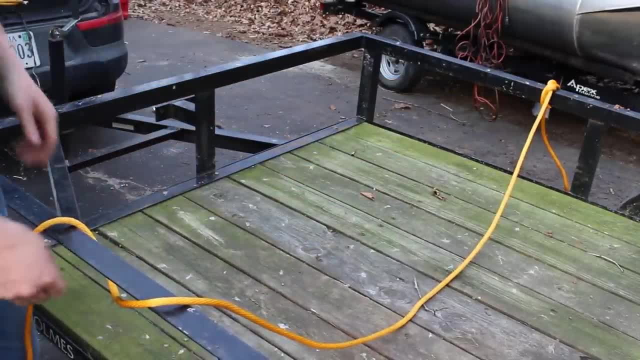 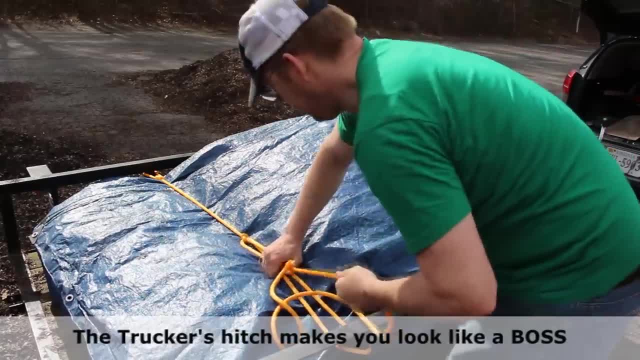 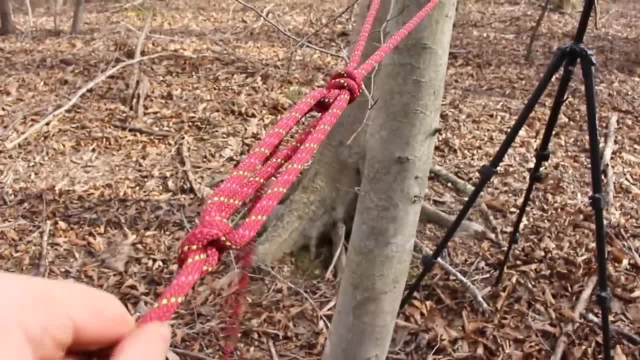 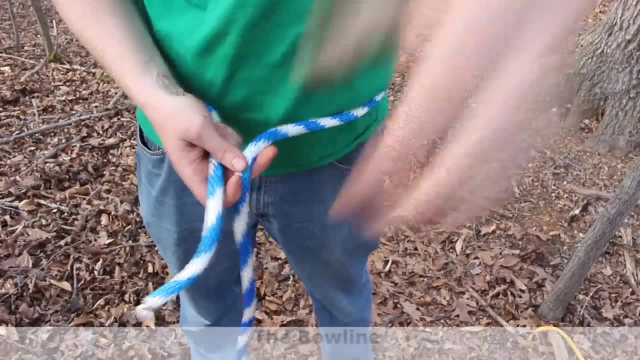 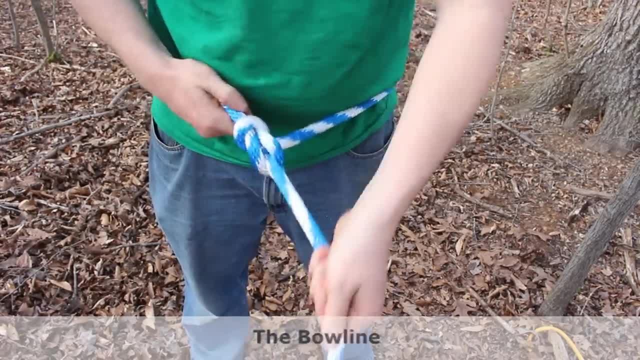 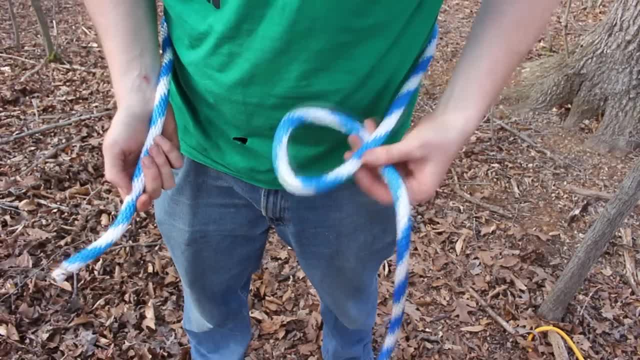 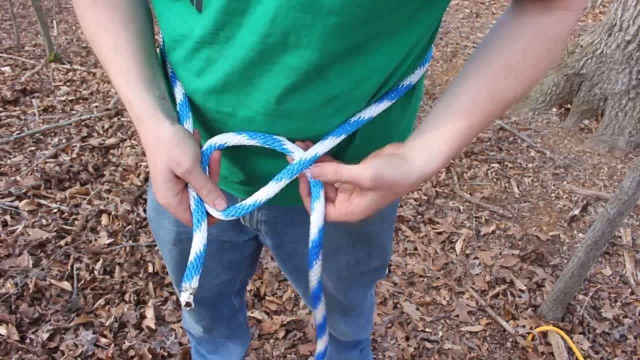 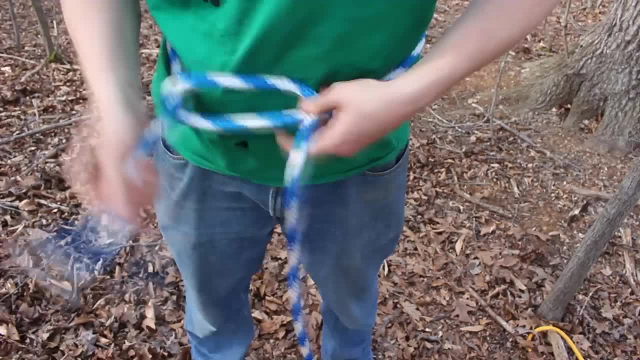 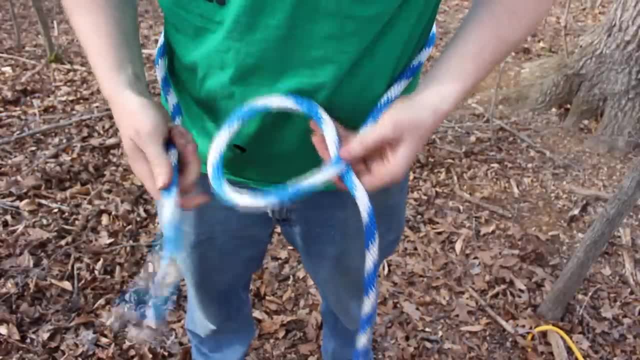 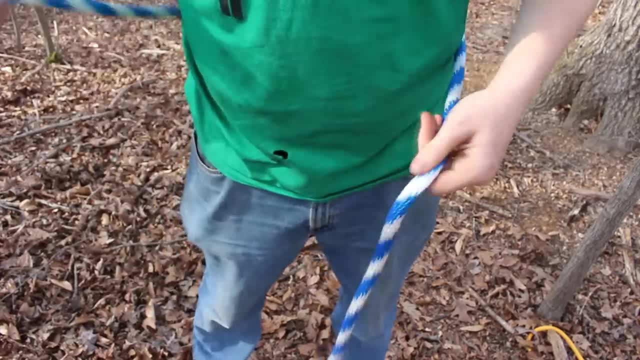 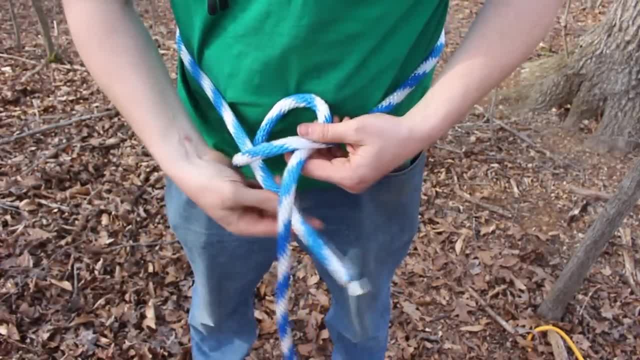 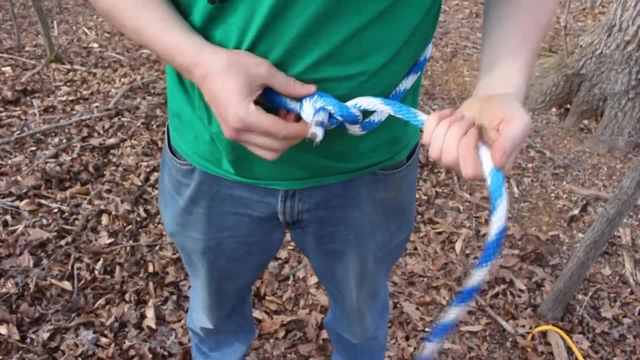 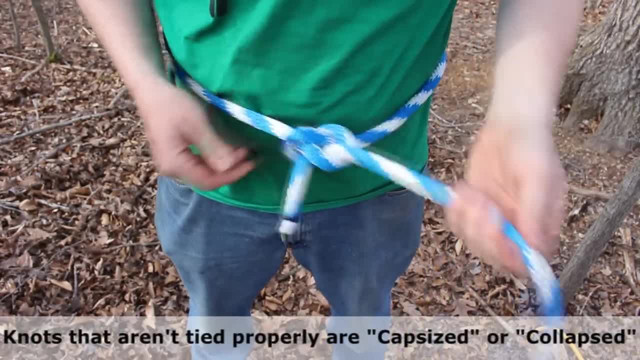 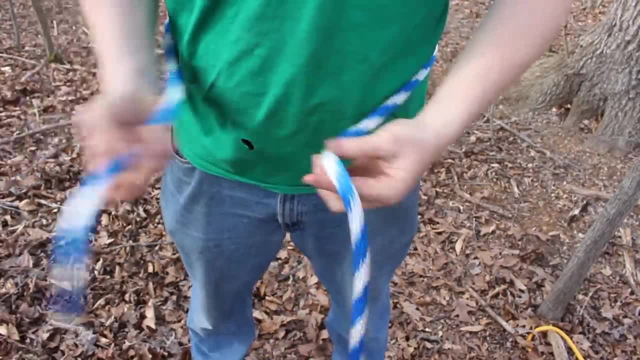 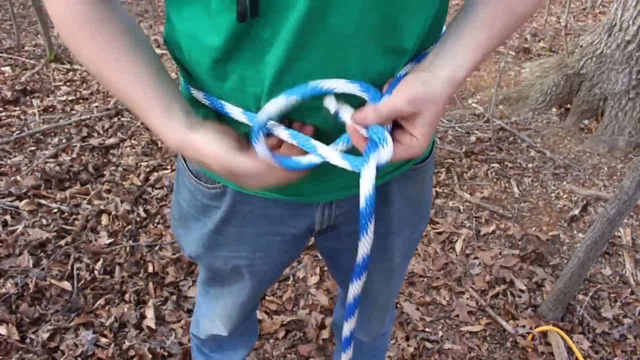 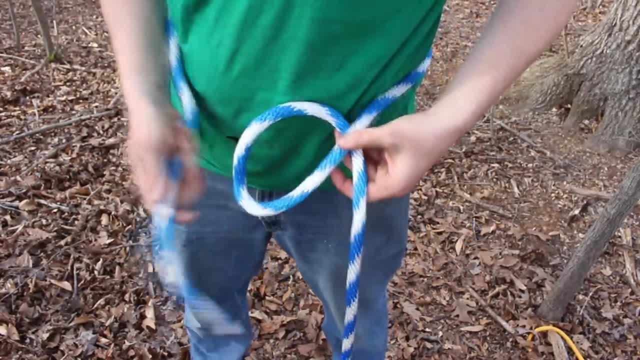 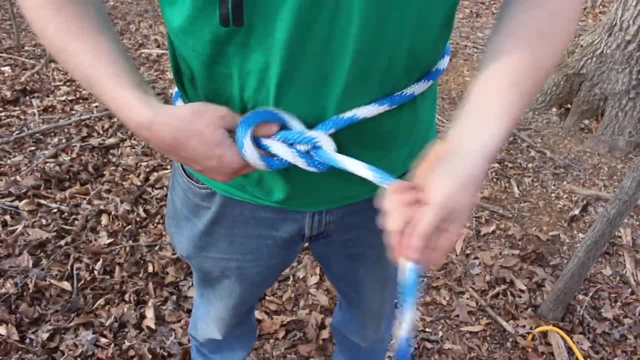 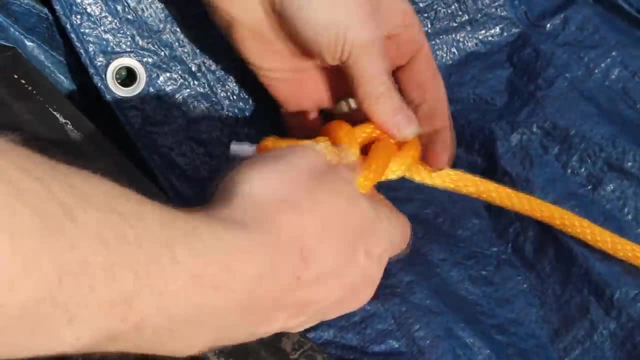 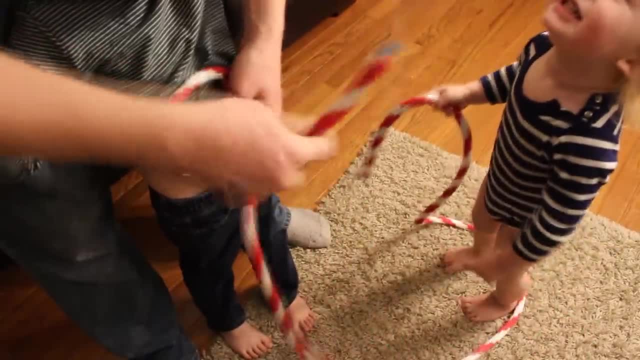 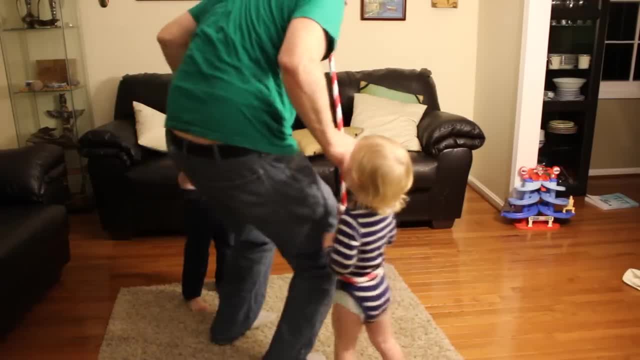 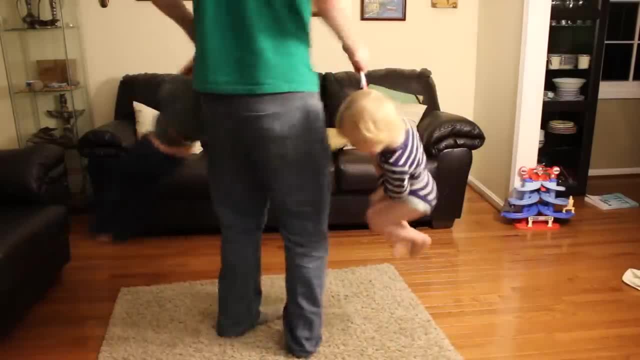 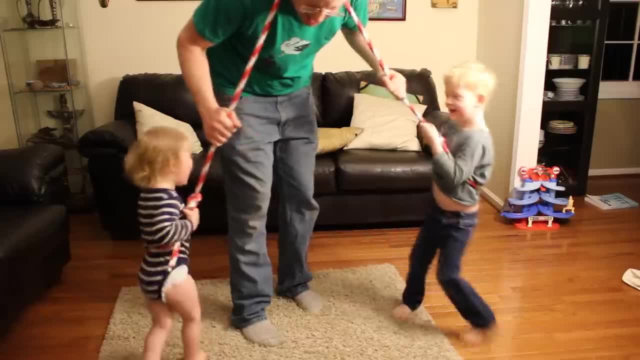 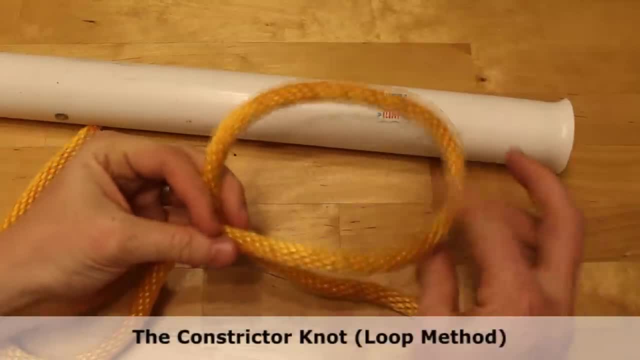 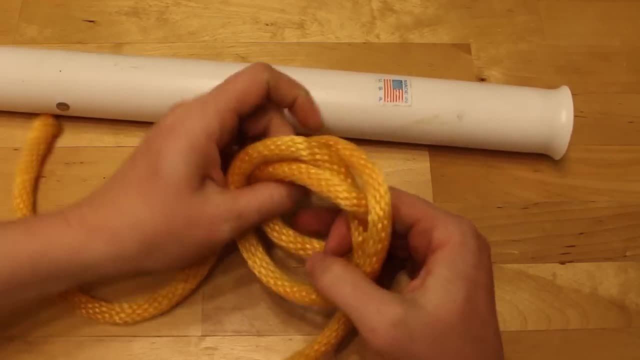 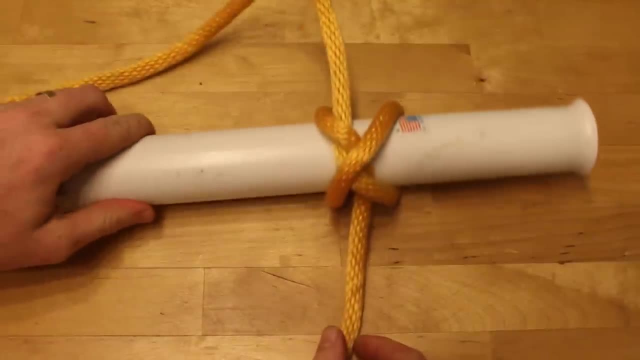 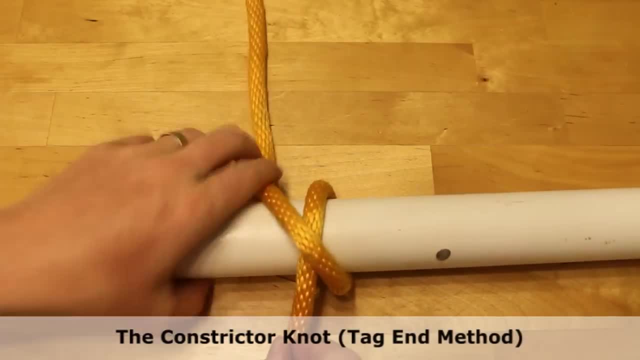 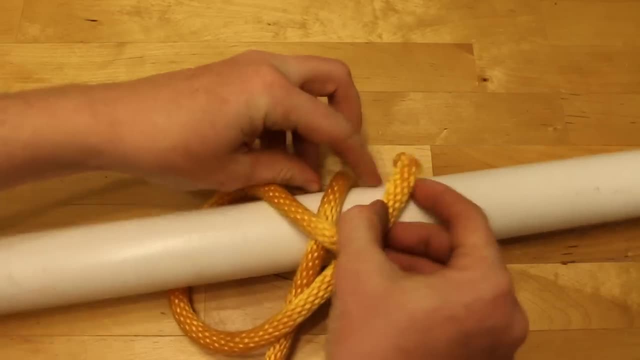 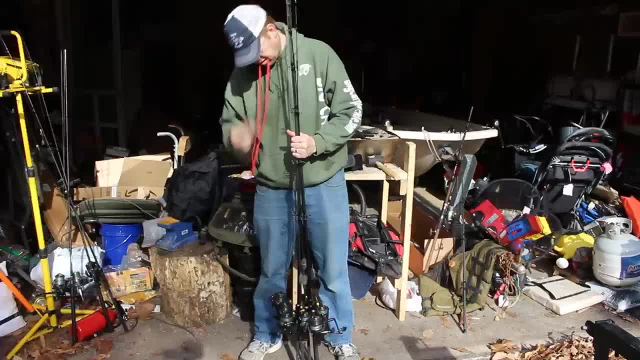 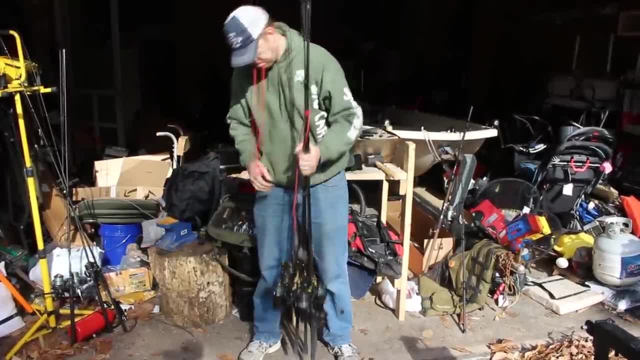 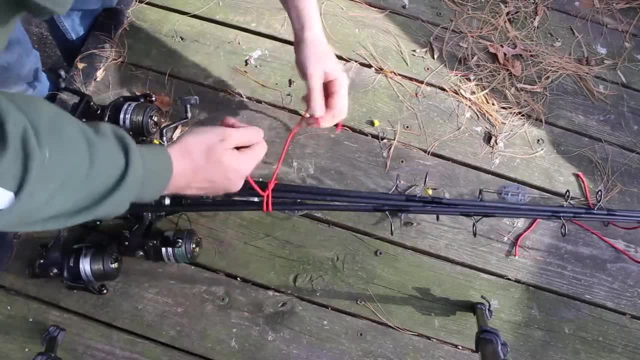 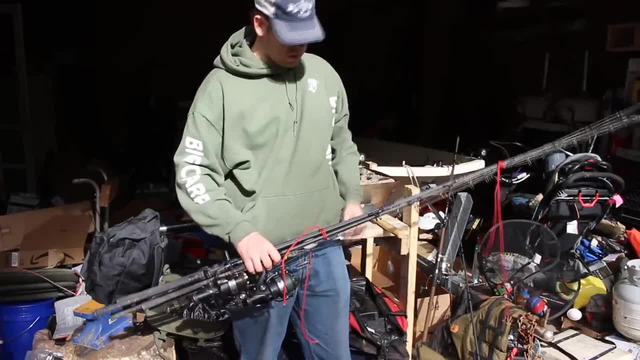 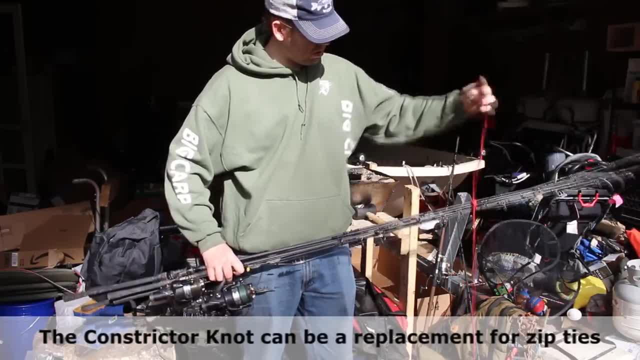 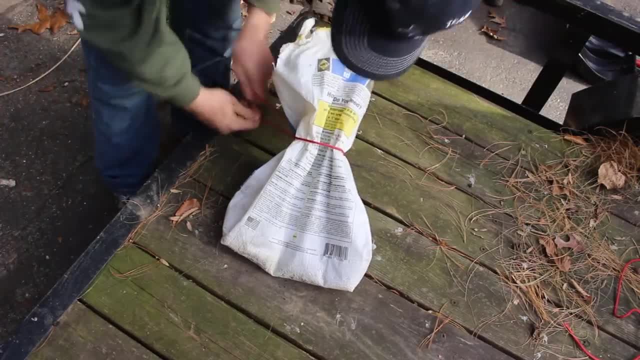 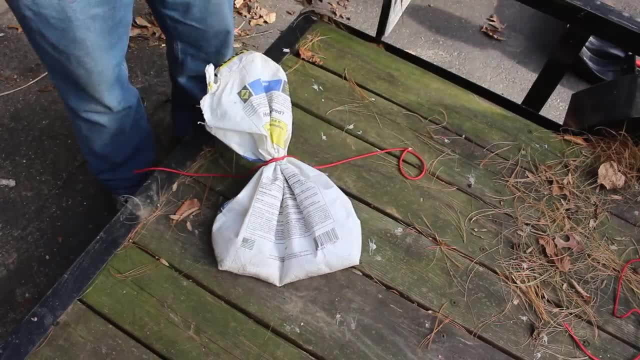 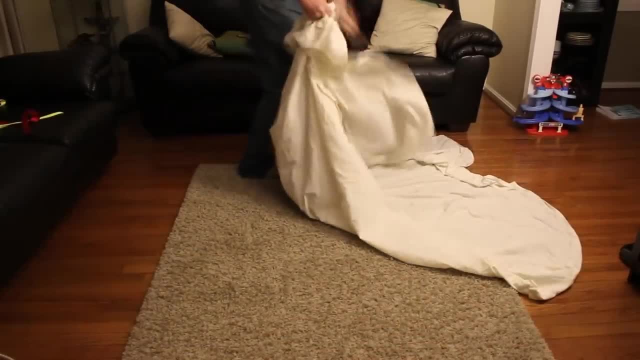 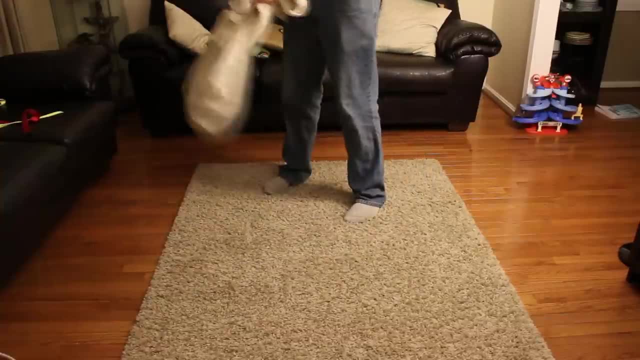 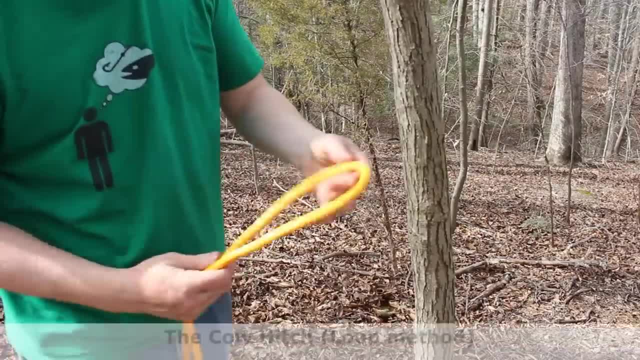 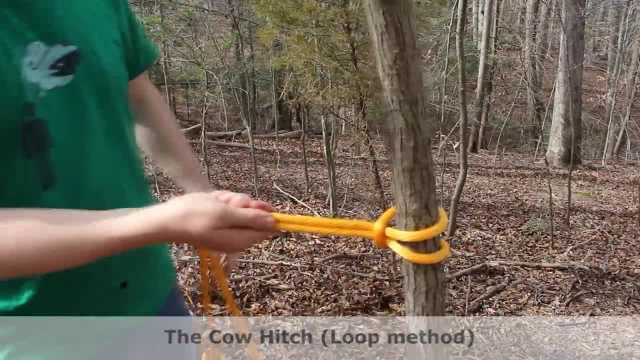 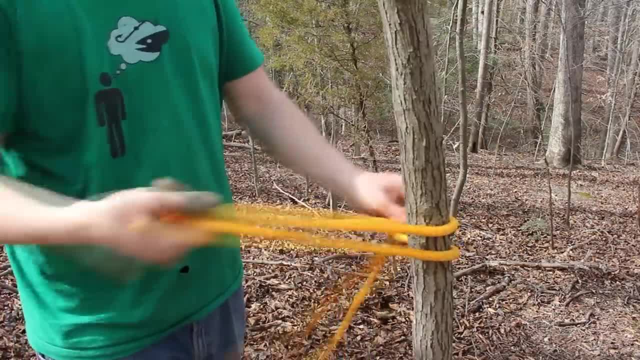 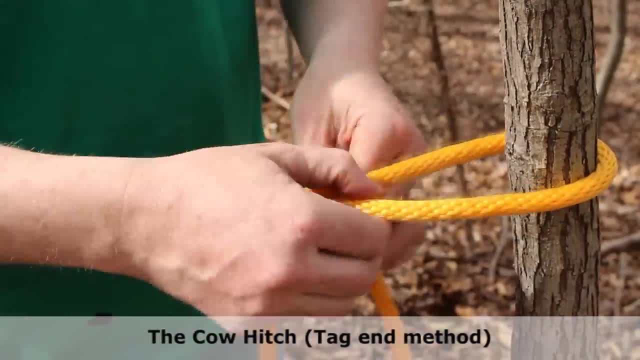 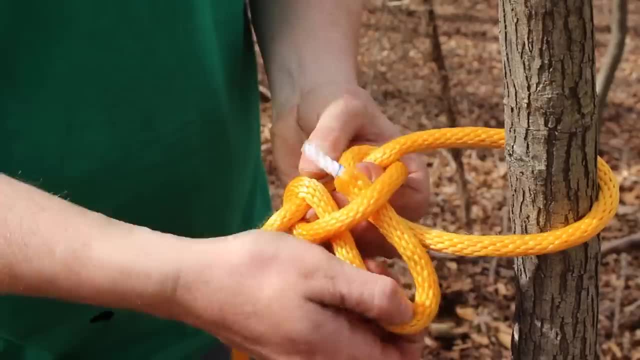 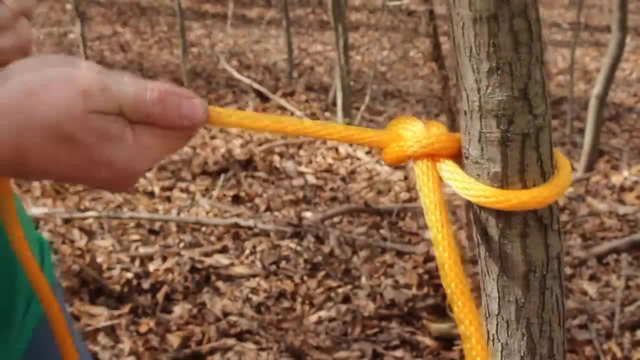 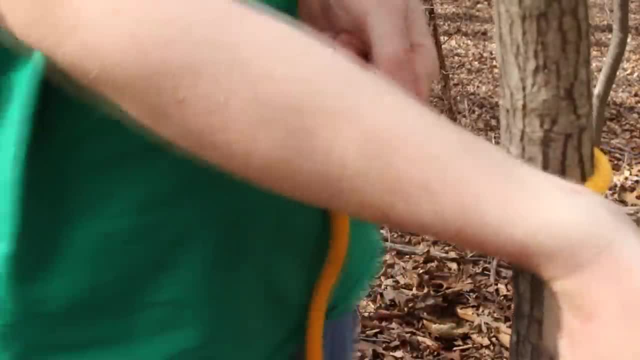 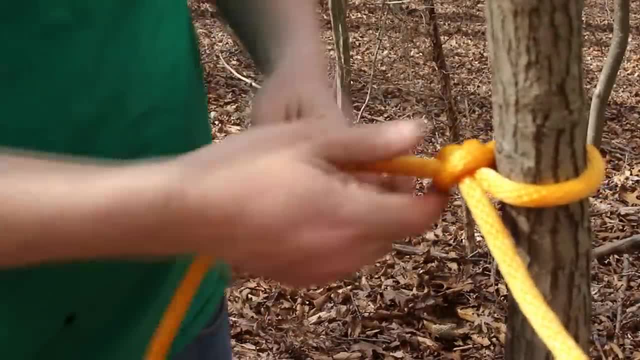 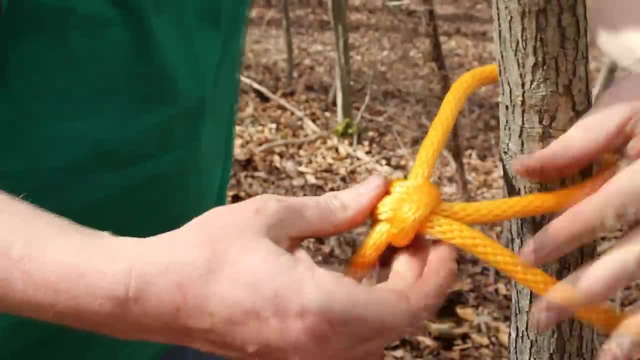 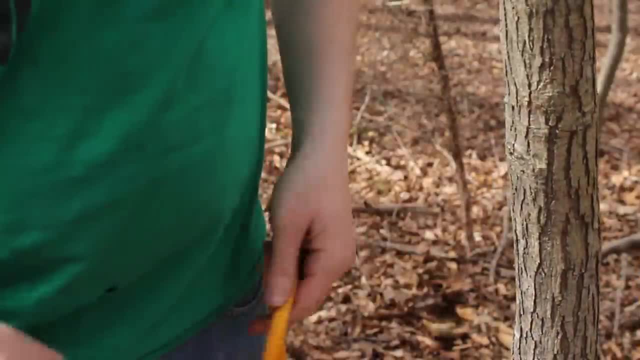 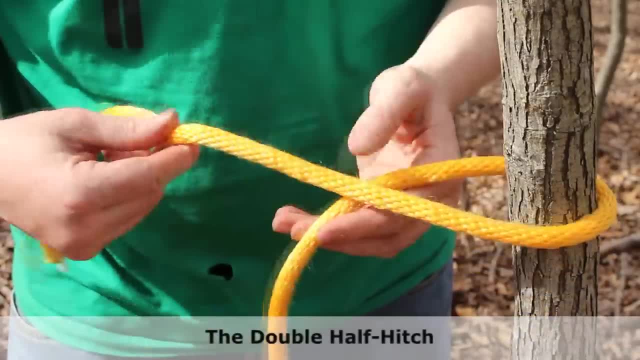 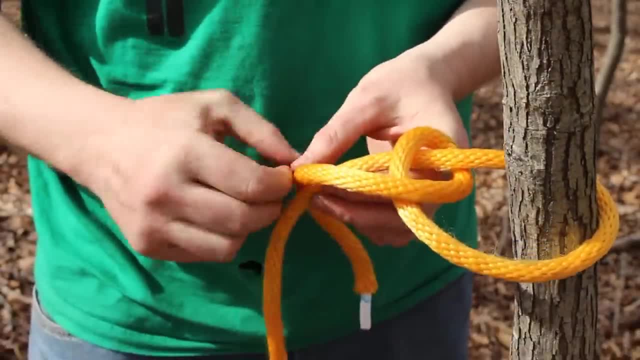 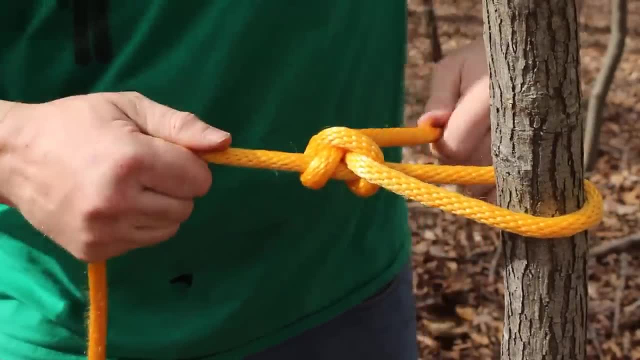 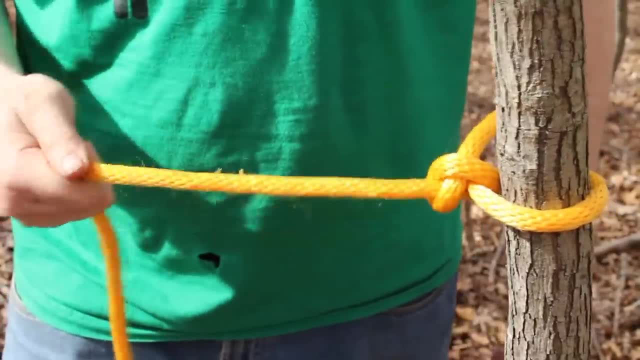 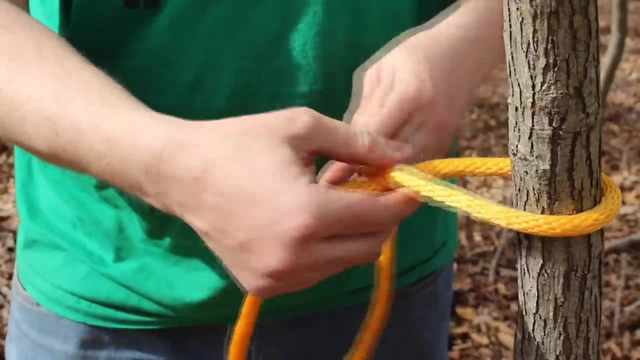 This knot allows you to adjust the length of a rope by adjusting the size of the loop at the end of the rope- as easy to untie as the cow hitch knot. the reason why i like this knot and why i'm including it is because you can do a quick release version of it, so it starts off just like the, the double. 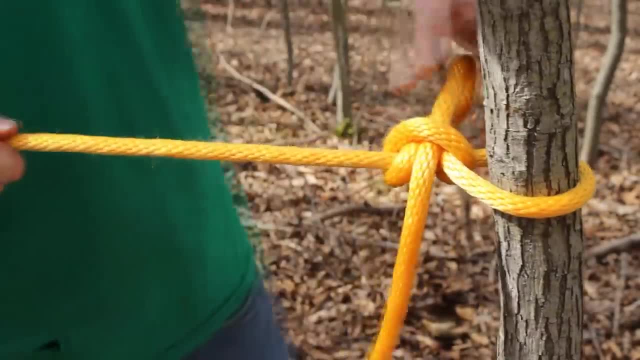 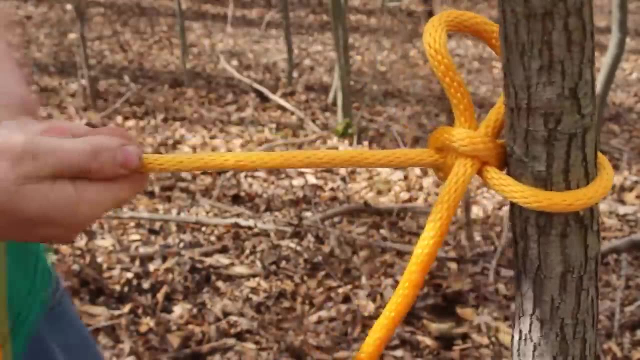 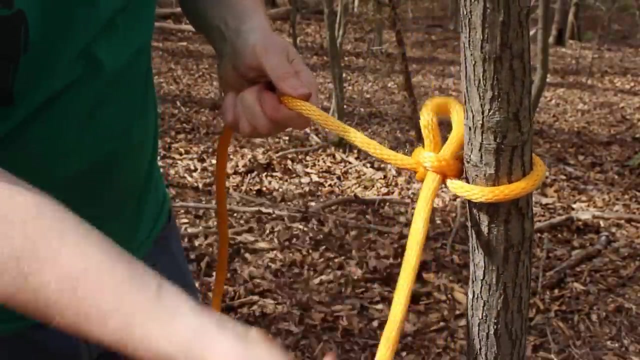 half hitch or the cow hitch knot. then you put a bite in it like this: cinch that up. and there you go, you've got a knot that cinches up and acts like the cow hitch knot, but then it's quick release, okay. so it's a nice little little version and if you want to be able to take a knot down really, 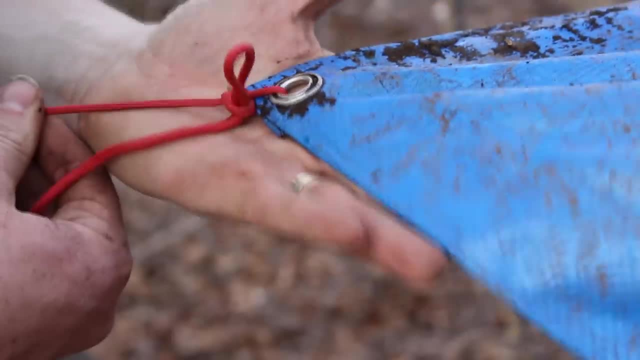 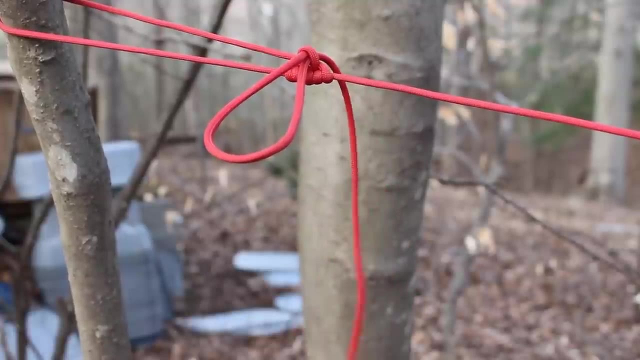 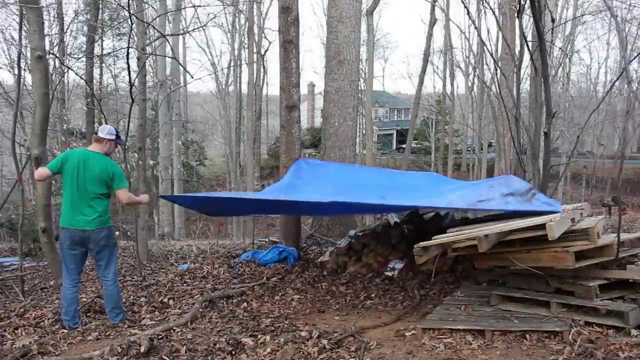 quickly. so when i use a fairman's friction hitch i tie this knot onto the other end of the line, so it's a quick release knot that's not adjustable. so one end i got the fairman's friction hitch and on the other end i've got the double half hitch with a bite and as you can see here, it 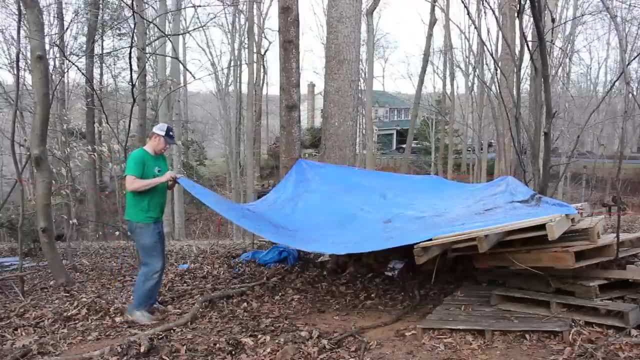 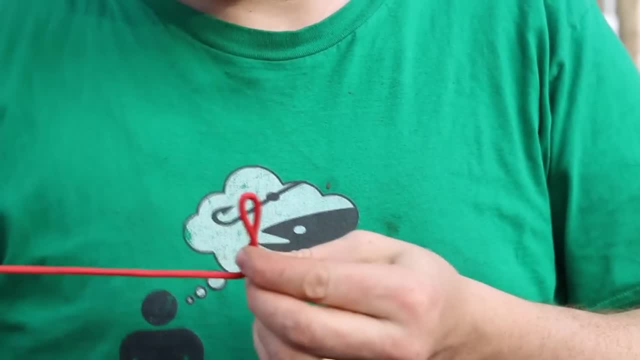 takes just seconds to untie it and get your rope back, so you can break down camp extremely quickly, very fast and efficient. okay, here's another little tip. it's not really a knot, but since we're on the subject of tarps, i thought i'd throw it in here. basically, pinch a little loop. 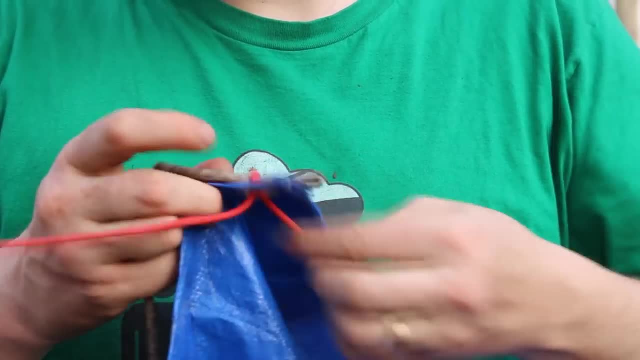 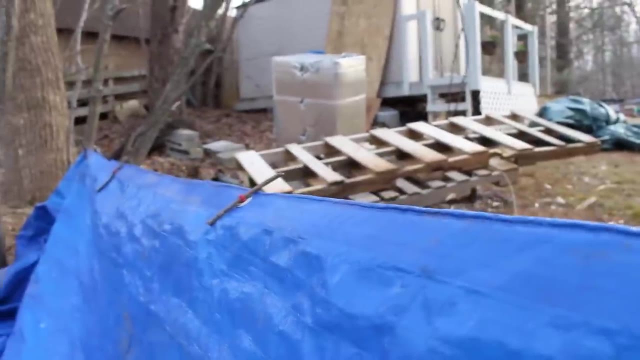 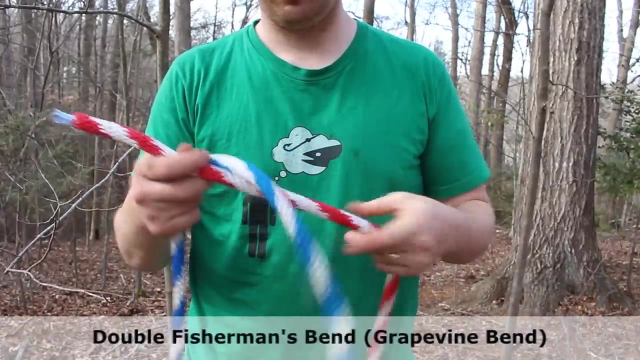 feed it through the grommet and then put a stick through it. trim it off. there you go. you've now attached your tarp to a ridge line, okay, and you can just go down the edge really fast- easy way to secure your tarp. so now let me show you the fisherman's bend, or the grapevine bend. 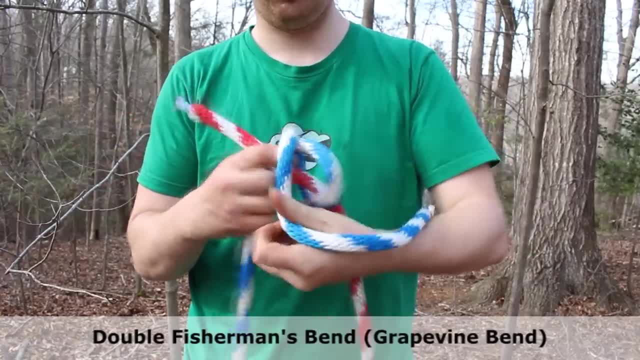 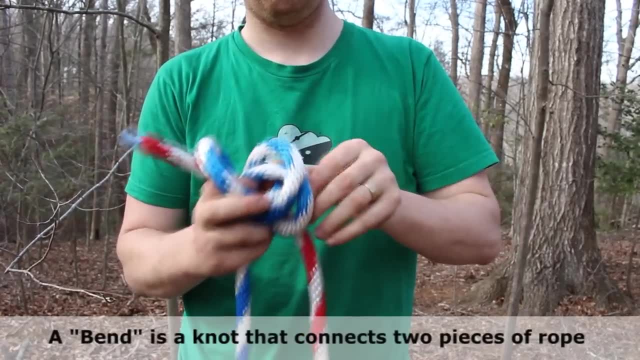 it's a great way of securing two ropes to each other, to tying dissimilar ropes or even different size ropes together. you tie this knot by putting what's called a strangle knot onto one of the ropes, and there's also similar to like a double overhand knot. 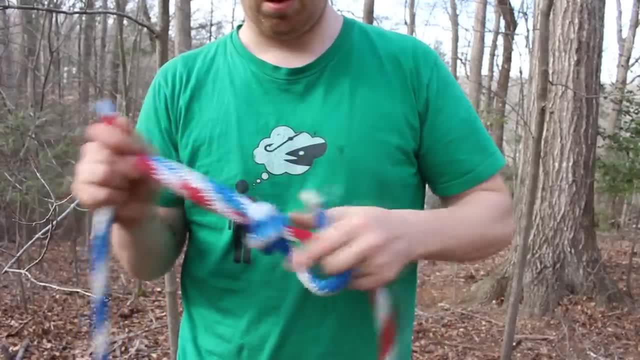 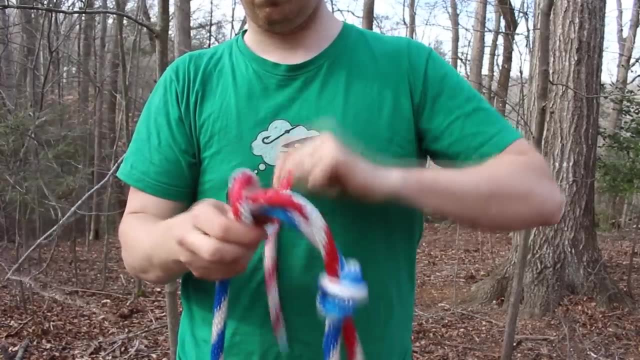 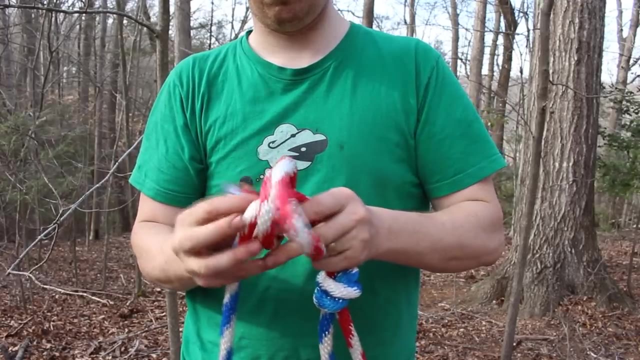 and you can see here. it's pretty simple, pretty fast to tie, not too complicated. that's what's the beauty of this knot. it's really simple. you just tie that strangle knot on one side and then the other rope to tie a strangle knot on the other side and when it's all done, the two knots will. 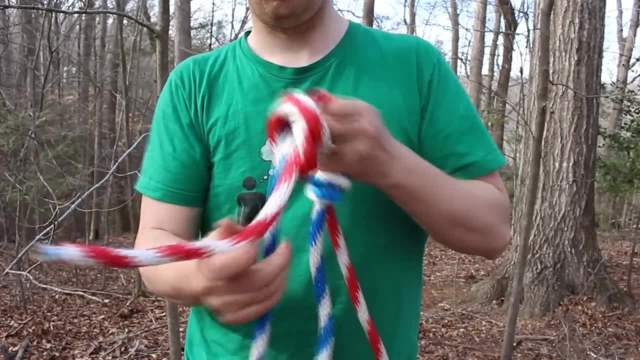 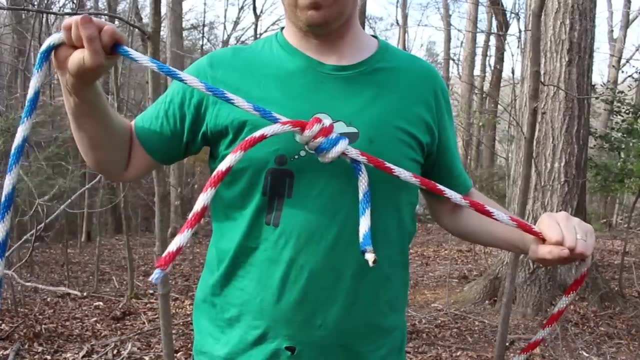 slide towards each other and they'll stop each other from going any further. this is a really strong way of joining two ropes and it doesn't take up a lot of rope to tie this knot. once you tighten that, it is not cupping off very easily. i barely pulled this together because i wanted 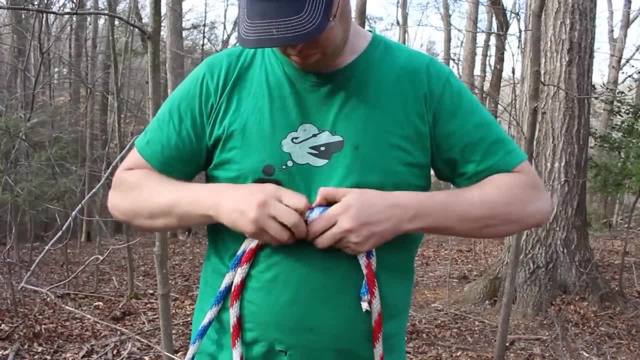 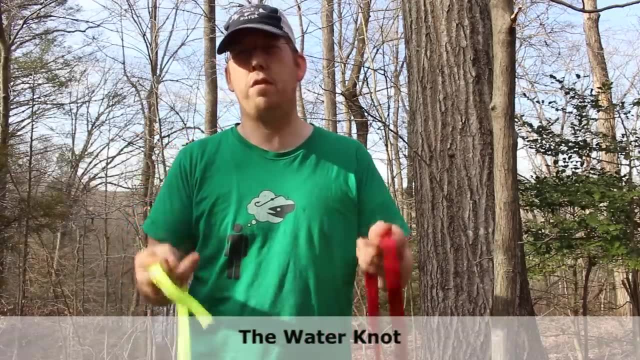 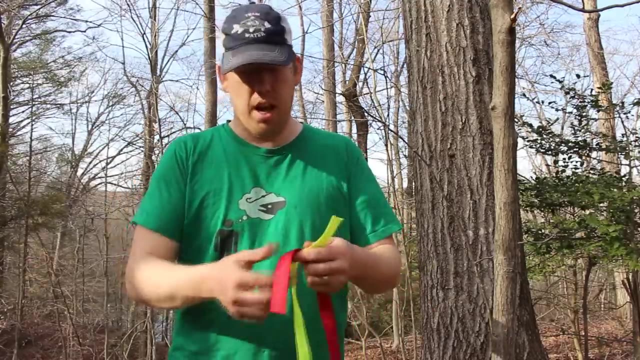 my rope back and i really had to get my fingernails out to get that knot undone. now here's another knot you need to know. it's the water knot. it is the knot for joining two pieces of nylon strapping together. it's super easy. you learn it once, you'll never forget it, and it's basically this: just make